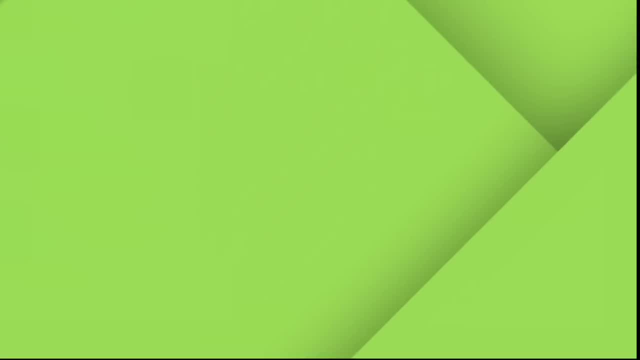 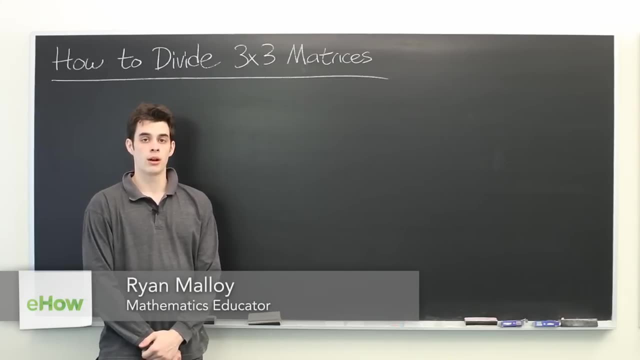 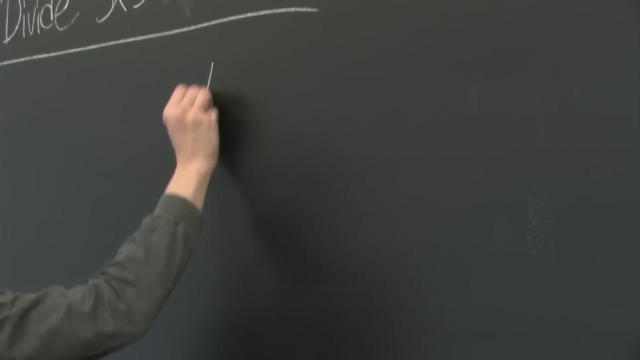 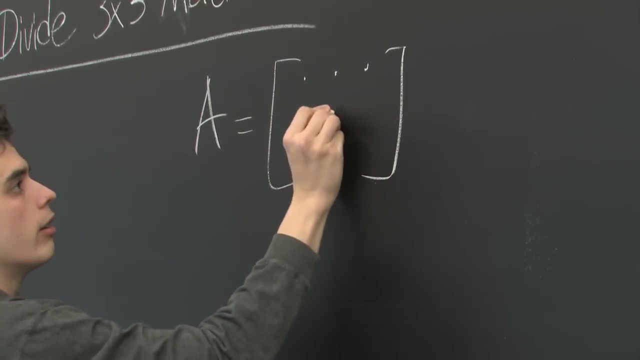 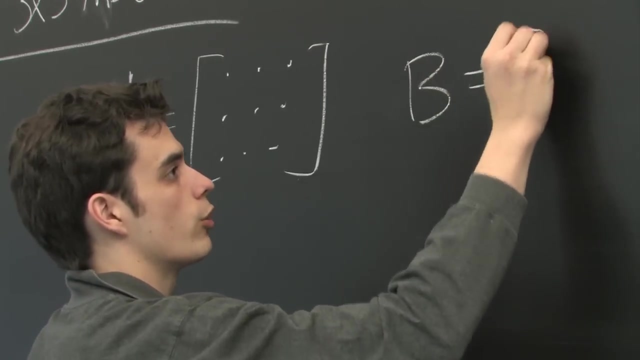 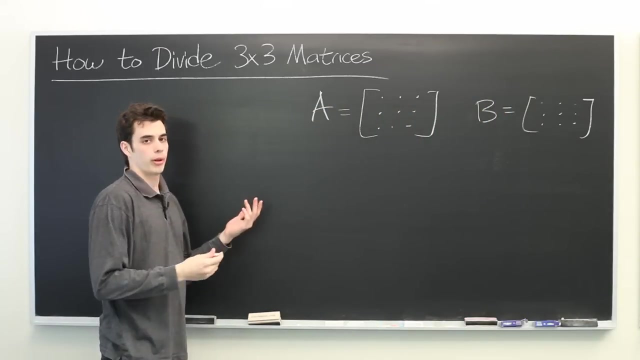 Hi there. This is Ryan Molloy here at the Worldwide Center of Mathematics. In this video we're going to discuss how to divide 3x3 matrices. So suppose that we have some matrix A which is 3x3. And suppose that we also have another matrix B, which again is 3x3.. Multiplying these: 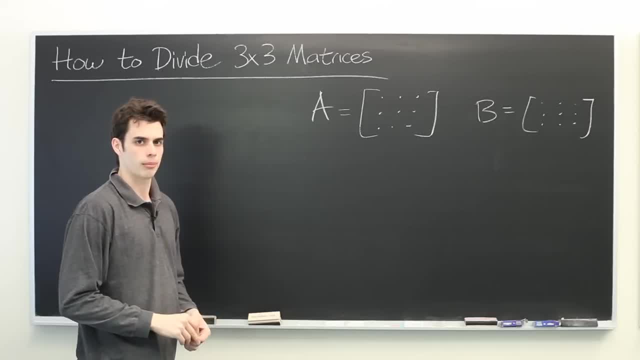 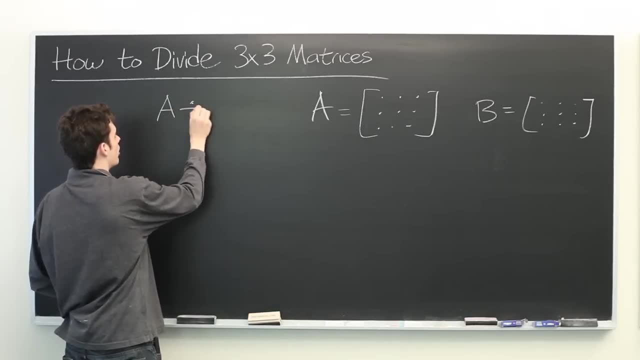 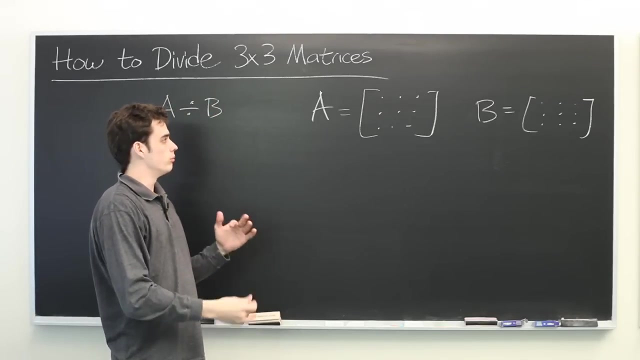 is fairly simple if you're familiar with matrix operations. But an interesting question is: can you divide these? Is there a natural way to come up with a formula for A divided by B? Yes Well, division of matrices. there is no direct way of doing it, But what one can do simply. 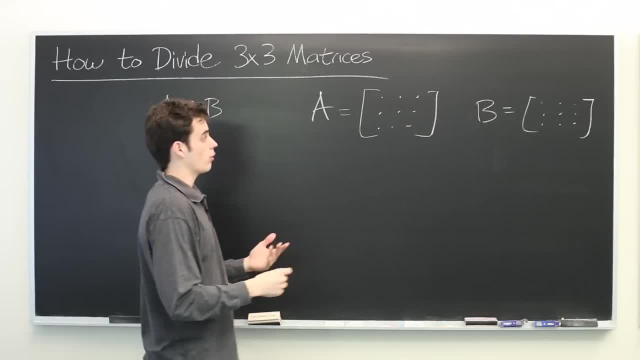 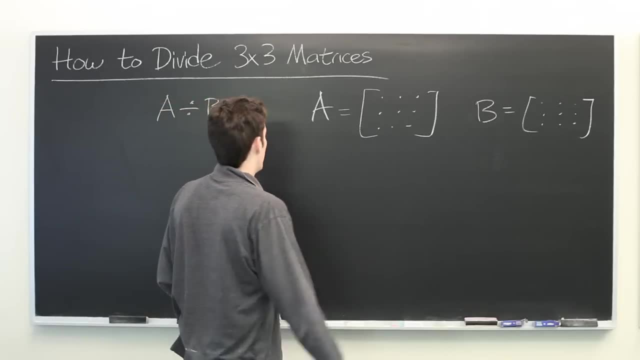 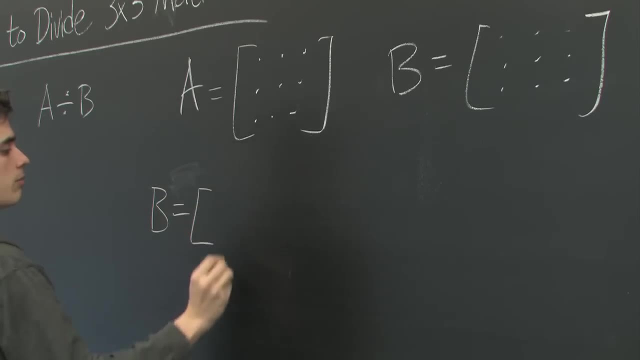 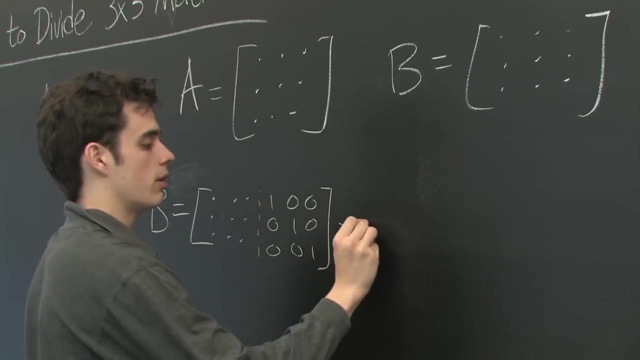 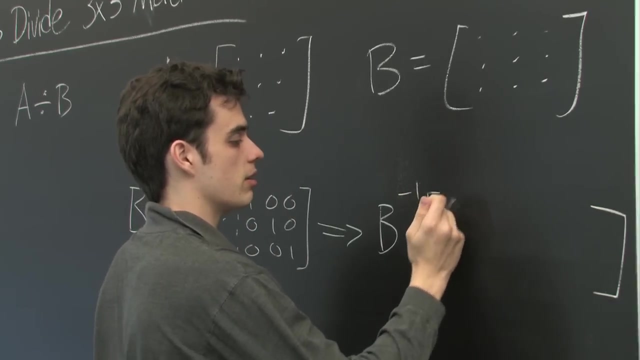 recall that division is the inverse of multiplication. In other words, in order to get A divided by B, we can simply multiply A by the inverse of B. So in order to do that, if we express B as an extended matrix With the identity matrix over here, We can get to the inverse By doing a series of row. 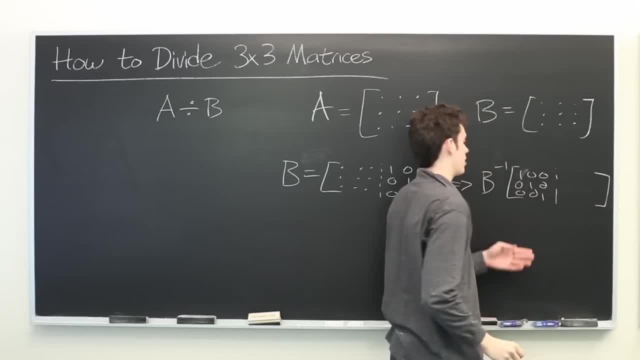 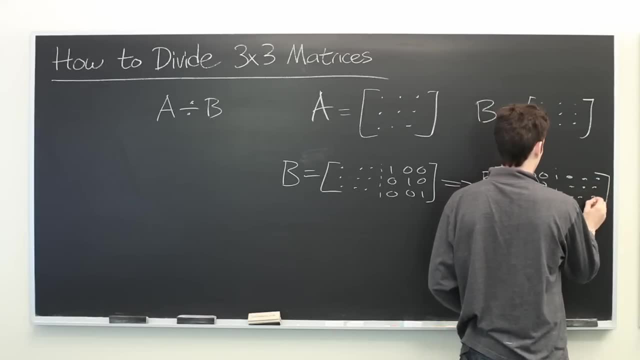 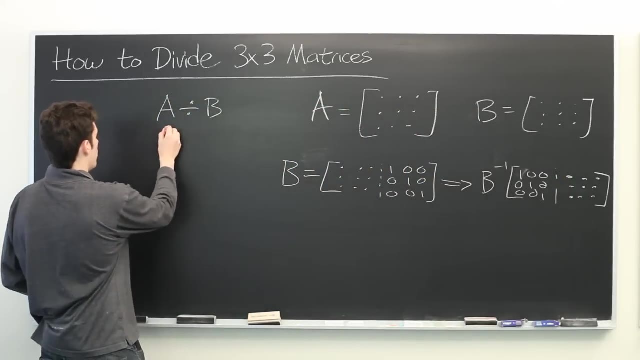 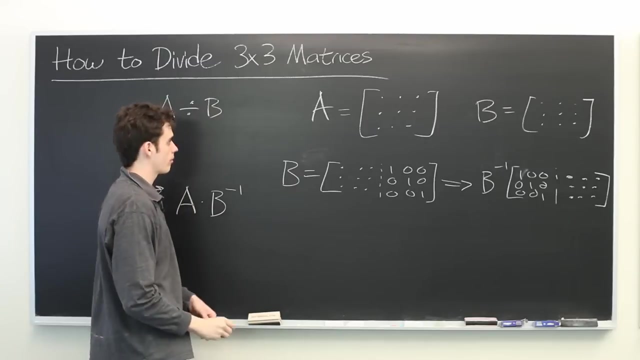 operations until the identity matrix appears on the left hand side, And then whatever we have here is B inverse. So once that is determined, this simply becomes A times B inverse, which can be done in exactly the same way that one would go about multiplying A times B And 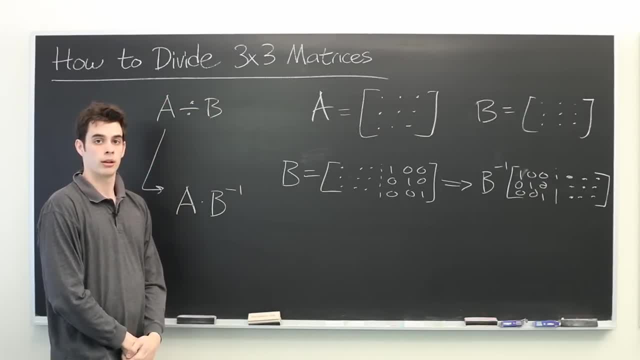 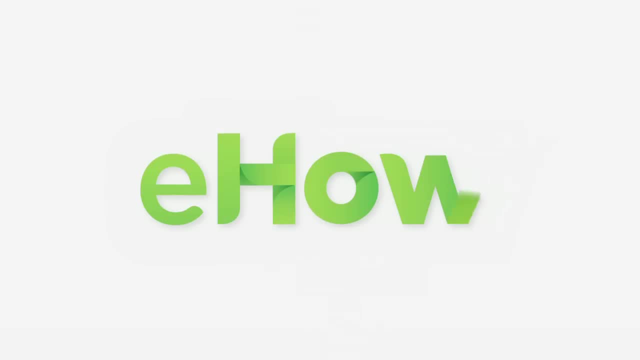 that's all there is to it. My name is Ryan Molloy and we've just discussed how to divide three-by-three matrices.